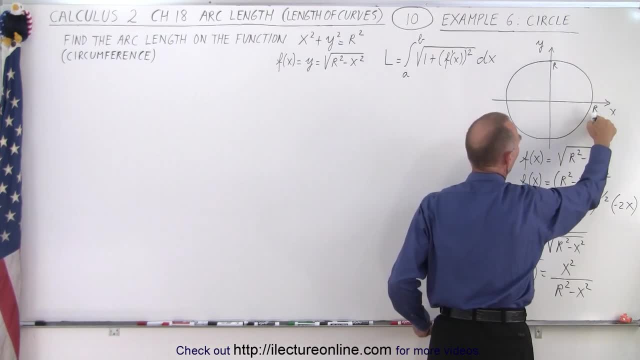 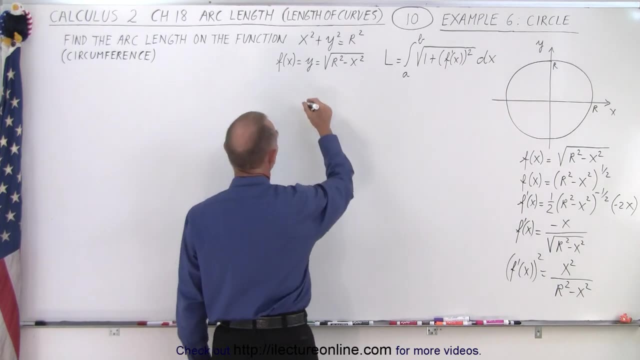 around the circle. let's just go one quarter. the distance from x equals r to x equals 0, 4, so we have the full length or the full circumference. so therefore we can say that the length is equal to 4 times the integral of going from x equals r to x equals 0. 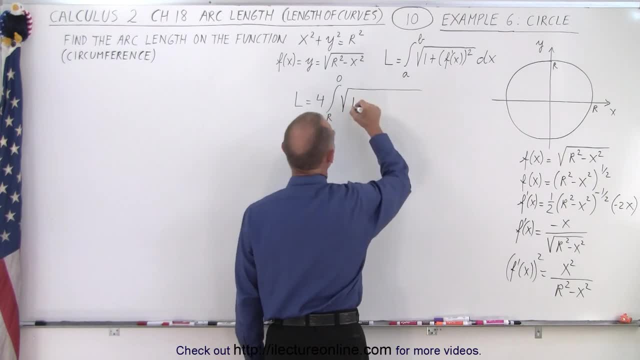 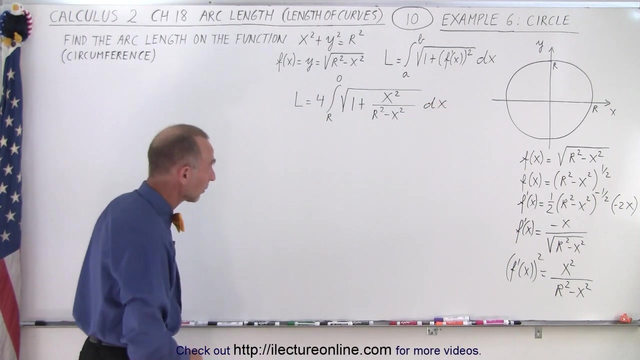 of the square root of 1 plus the derivative of the function squared, which is what we have right here. so it would be x squared divided by r squared minus x squared times dx. now, at first you take a look at that and go, wow, how do I integrate that? but we can simplify that algebraically. we can put: 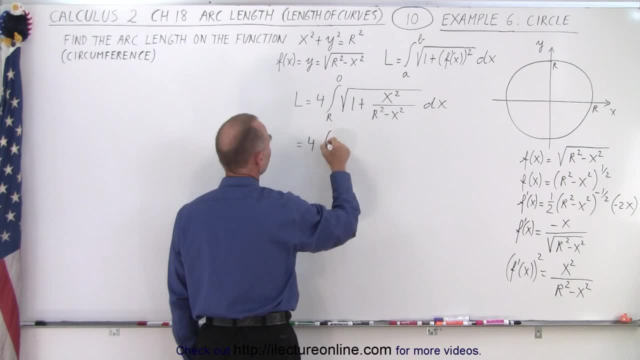 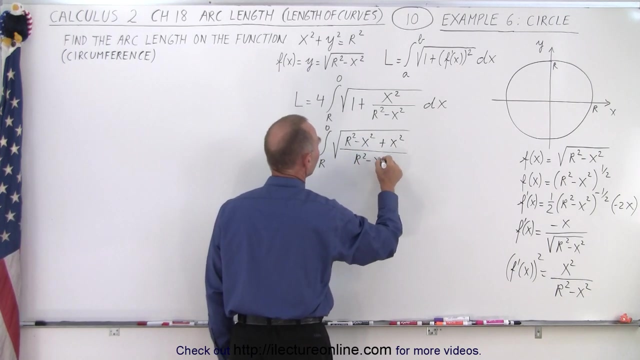 it all over the common denominator. so this is equal to 4 times integral from r to 0 of the square root of now. this becomes r squared minus x squared plus x squared divided by the common denominator of r squared minus x squared. of course, if I divide this by this, I get to 1 again, so it's 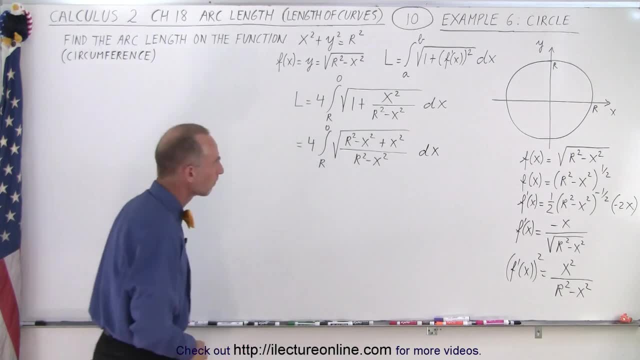 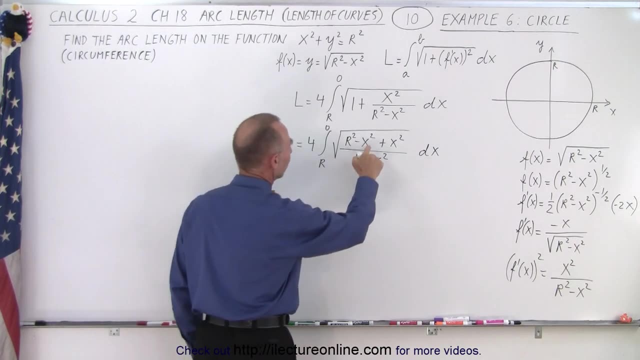 the same thing times dx. so now let's see here what can we do next? well, notice that the x's cancel out. so this becomes equal to 4 times the integral of, from r to 0 of the square root of r squared, divided by r squared. 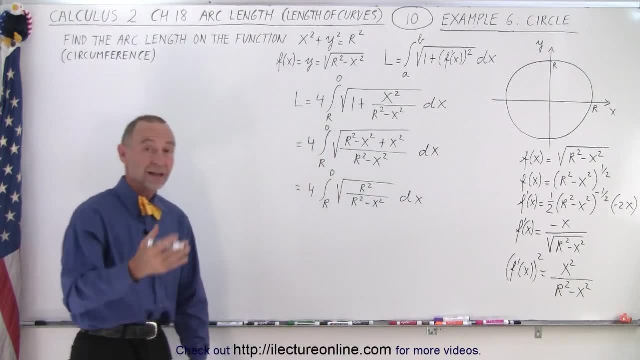 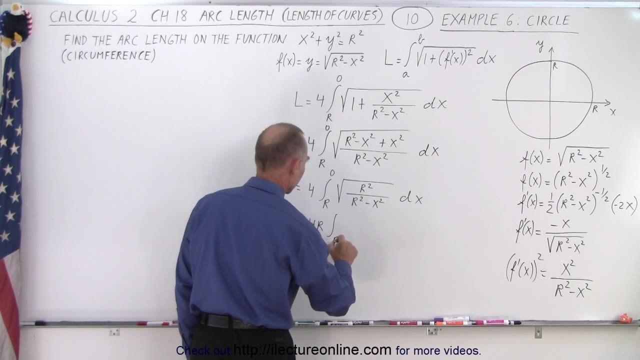 minus x squared times dx. and now we can factor out the r squared in the numerator, so we'll bring that over here. so this is equal to 4r times the integral from x equals 0 to x, x equal r to x equals 0, and then we have the square root of 1 over r squared minus. 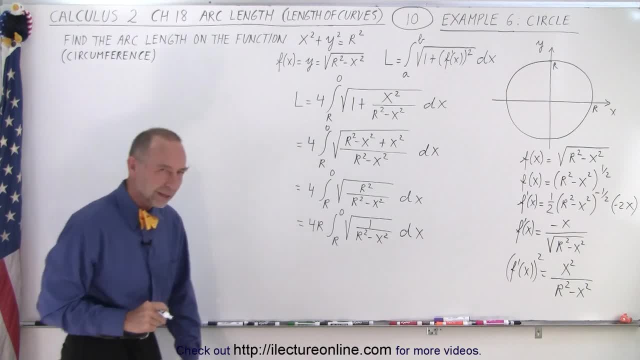 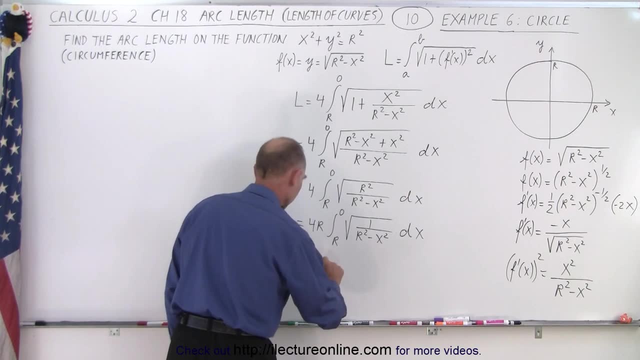 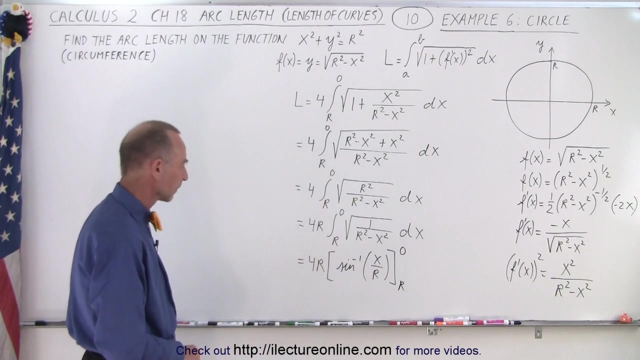 x squared times dx. and now we recognize the integral, because the integral of that that would be equal to the inverse sine. so this becomes equal to 4r times the inverse sine of, and that would be x over r. this, evaluated from x equals r to x equals 0. all right, let's come up here to evaluate that. so that means that the length is. 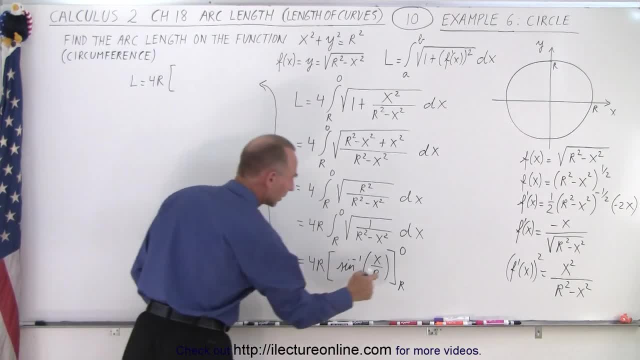 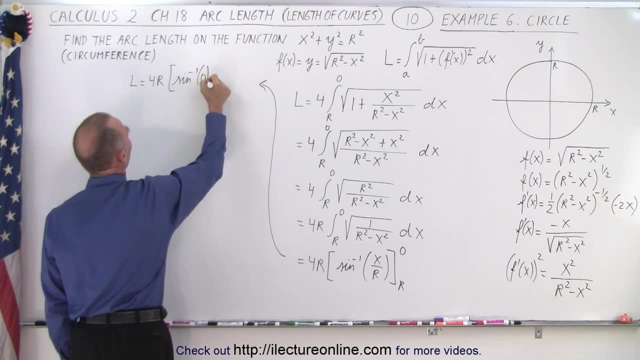 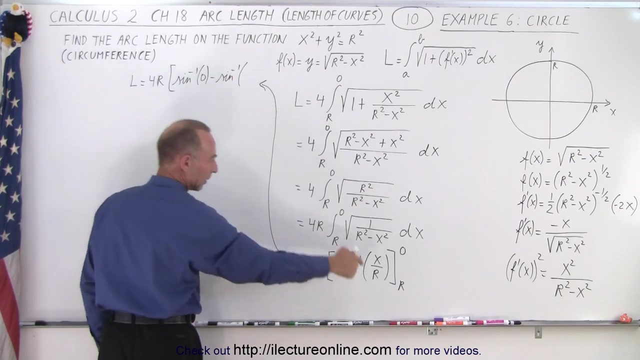 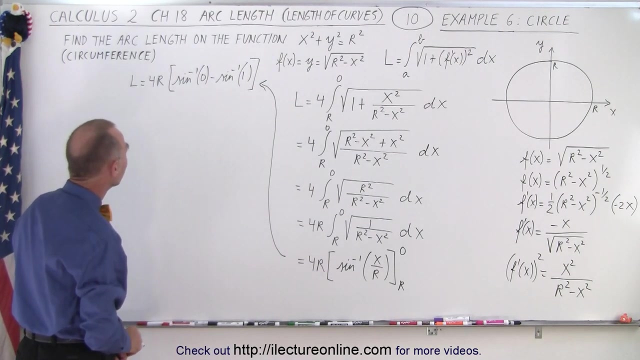 equal to 4 times r times. when plugging the upper limit, we get the inverse sine of 0, so the inverse sine of 0 minus when plugging the lower limit, we get the inverse sine of. that would be r over r or 1. okay, so when is the inverse sine when? what's the angle? when the inverse sine equal to 0? well, when 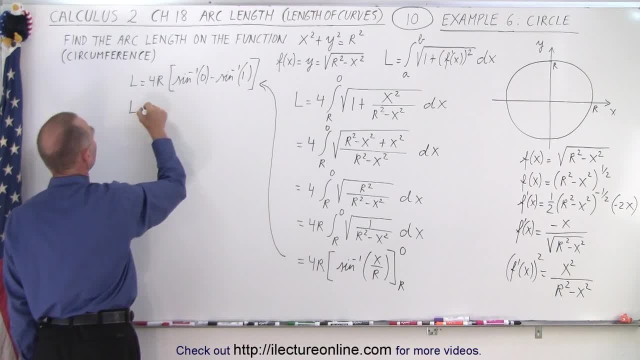 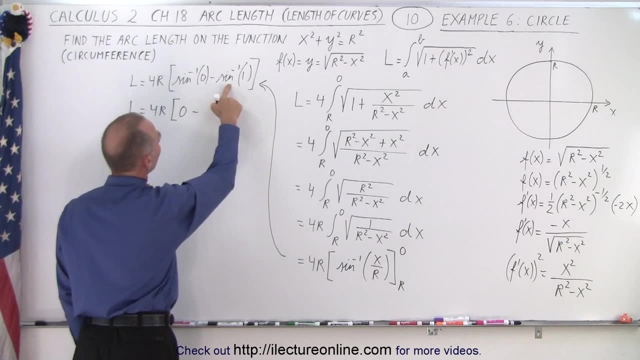 sine equals 0, that means the angle is 0. so l equals 4r times 0 minus. and then here with when the sine is equal to 1, well, that's equal to pi. so it looks like pi halves, right, that's 90 degrees. when the 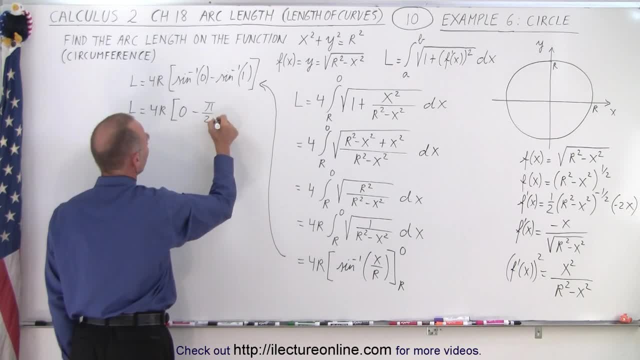 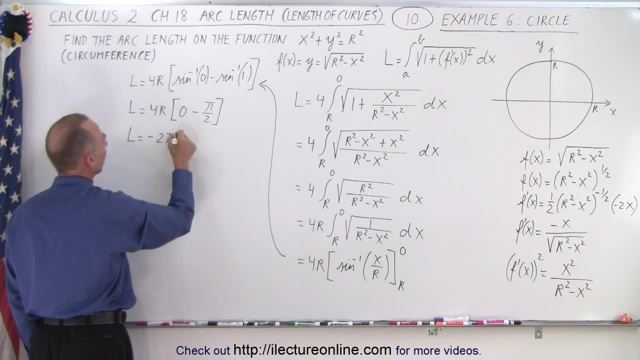 when the angle is 90 degrees, the sine is equal to 1, and then when the sine is equal to 1, the angle is 1, so pi halves. so here, the 4 divided by 2 is 2, so this gives us l is equal to minus 2 pi r. well now. 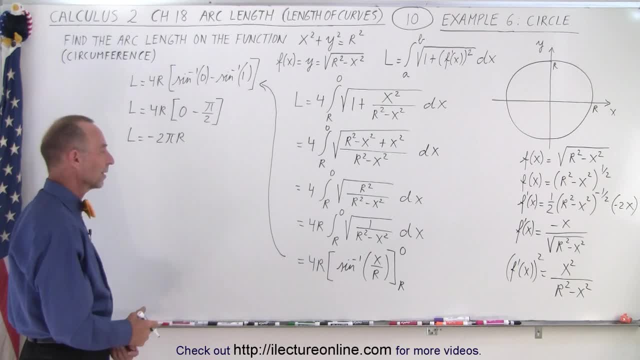 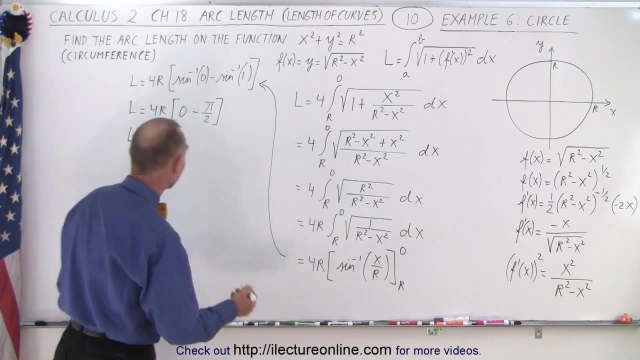 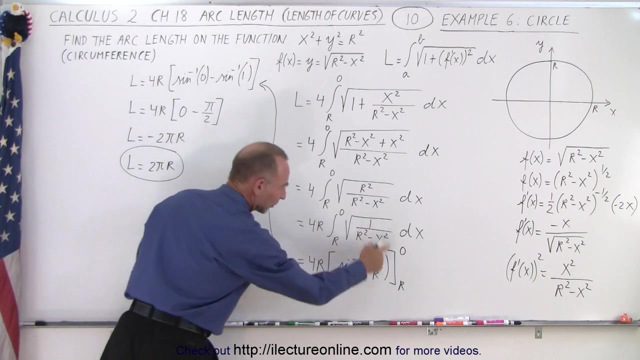 you say: well, you got a minus sign. how can that be? well, it turns out that i use the limits going from r to 0. if i then change the limits from 0 to r, i get the positive value. so essentially we can say that l is equal to 2 pi r if we plug the limits in the correct way, put r up there and 0 down there. 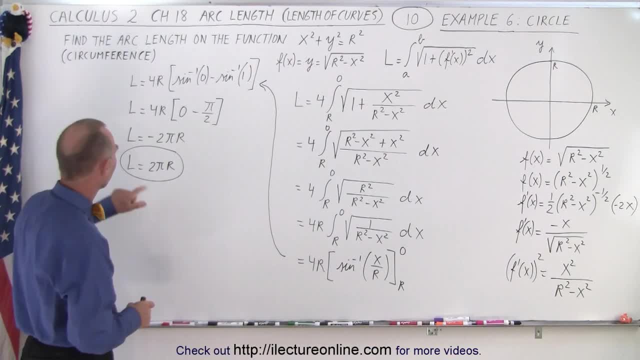 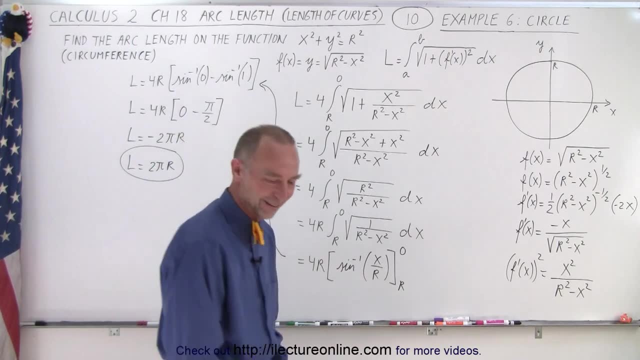 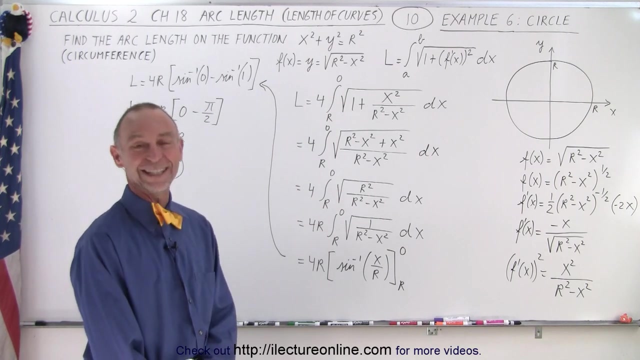 so that would be the same thing. wow. and so therefore, the length is 2 pi r, which is, of course, the circumference of the circle. no, no, no, no, that's not. i'm sure they did not figure it out like that initially. that would be the hard way to do it.